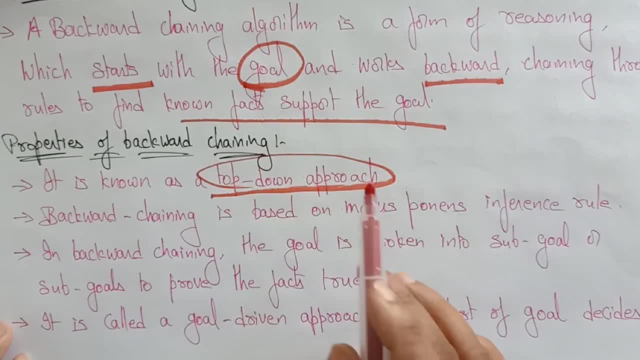 chaining. This is also known as the top-down approach, whereas the forward is the bottom-up approach, but bottom-top approach, and whereas backward chaining is the top-down approach, A backward chaining is based on the modest bonus inference rules. In backward chaining the goal is broken into sub-goals. So first, whatever the goal that we are reached. 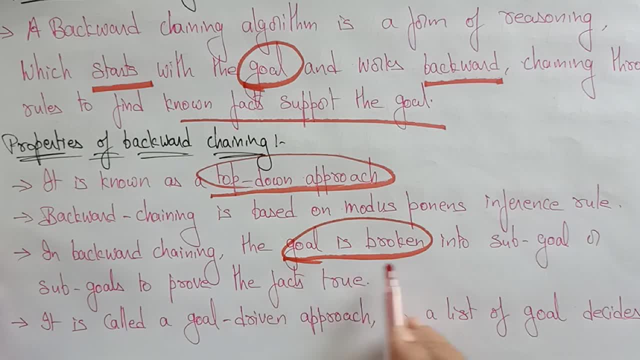 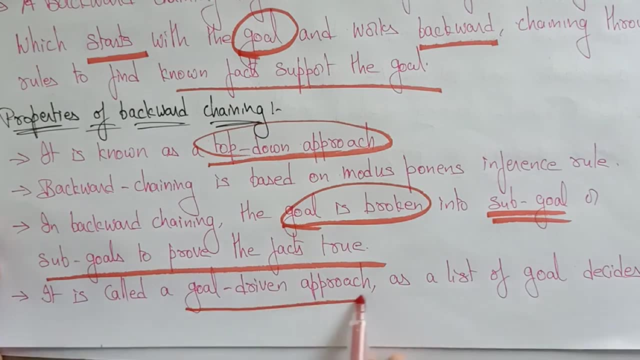 so with the help of the goal, we are reaching to the initial state. So the goal is broken into sub-goals or sub-goals to prove the facts true. So it is also called as goal-driven approach, whereas the backward chaining is the data-driven approach, because with the help of the data we are reaching. 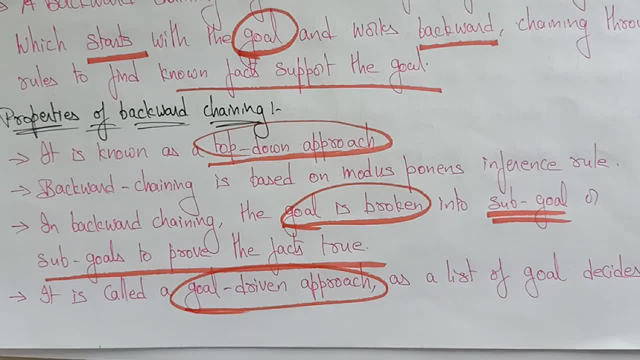 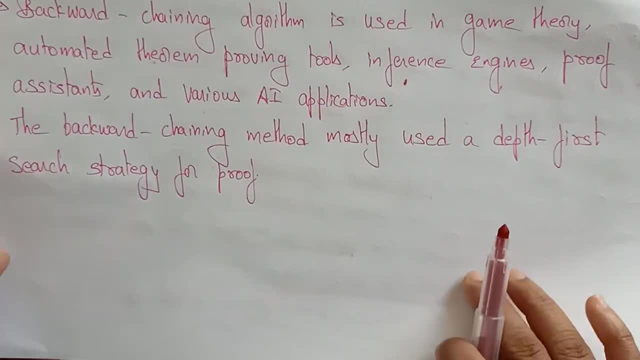 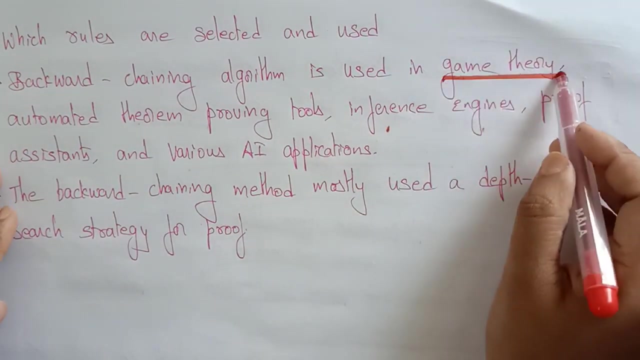 the goal, but in the backward chaining, with the help of the goal, we are reaching to the data. So that's why it is a goal-driven approach, As a list of goals decide which rules are selected or used. Backward chaining algorithm is used in a game theory, So it is used in game theory automatic. 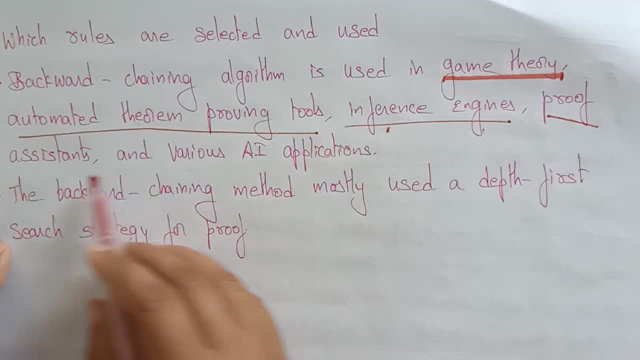 theory, proving tools, inference engines, proof assistance and various application, artificial intelligent applications. So the backward chaining is used in these different concepts: game theory, various artificial intelligent applications, proof assistance, inference engines. The backward chaining method mostly used a depth first search strategy for the 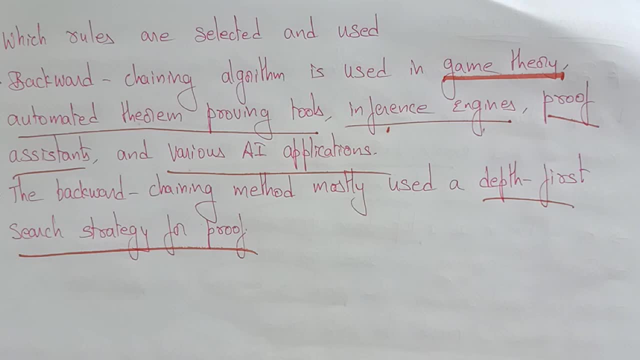 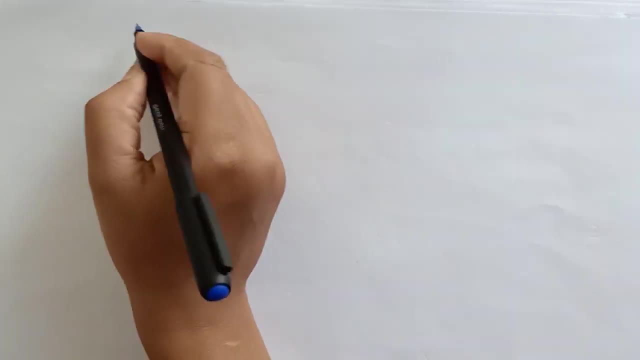 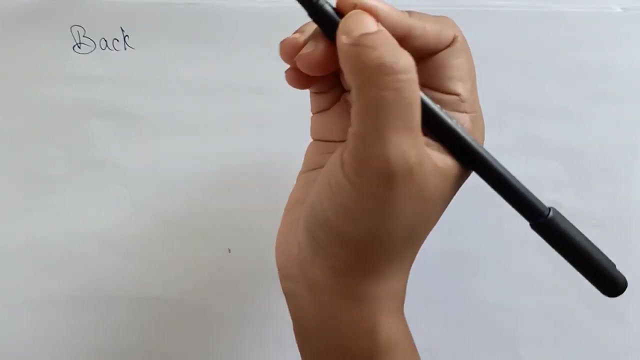 proof. So this is the theory part of the backward chaining. Now let's see the example. So, just like the forward chaining, the backward chaining example. let's see. So I am taking the same example. what is the same example? the goal state is a Z and the termination condition is: I have 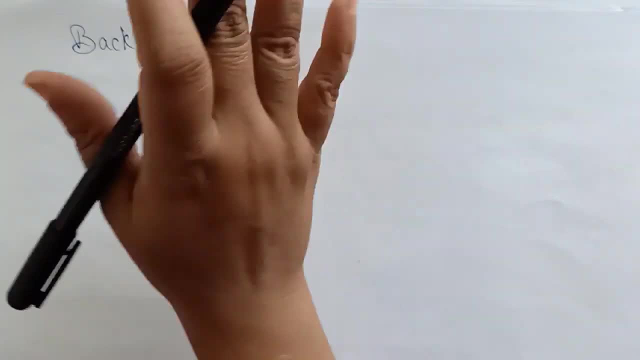 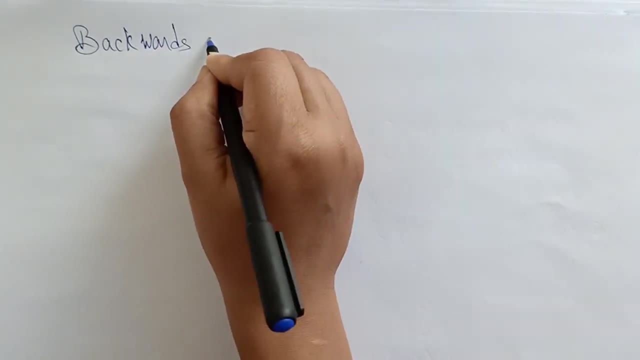 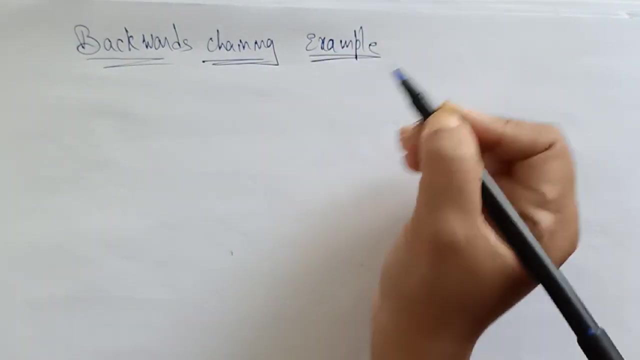 to stop whenever I reach the means. that means the thing here is a goal, state Z, and some facts are that there. So, with the help of the goal state, I am starting the chaining process, The backward chaining example. Okay, so now let's see. So what are the facts? The facts initially. 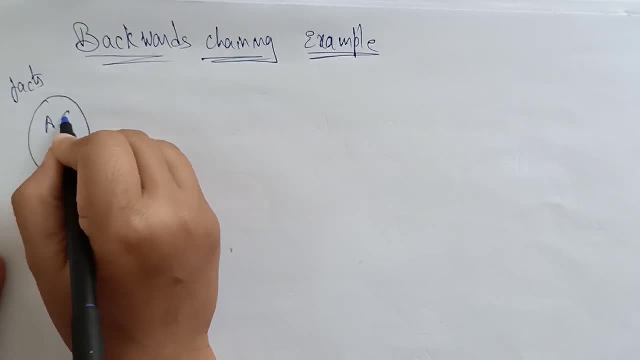 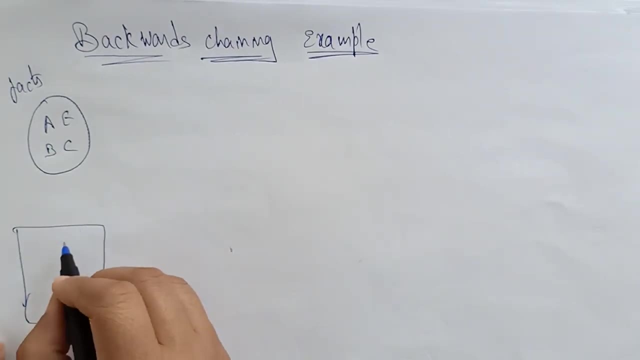 the facts the database contains. they are given as A, E, B, C. Okay, so now the rules. the rules that are implemented here is F and B implies Z. The same example I am taking: C and D implies F and A implies D. 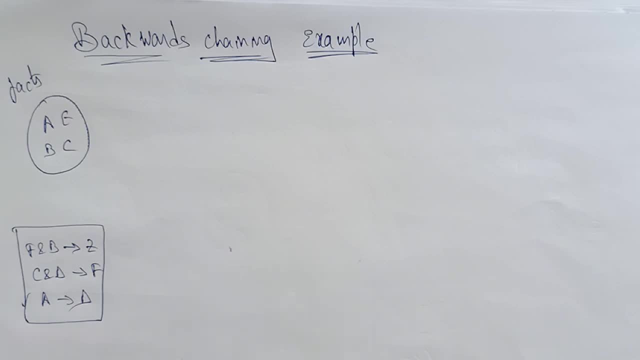 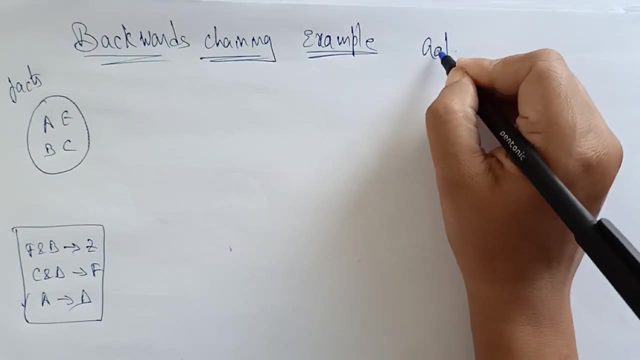 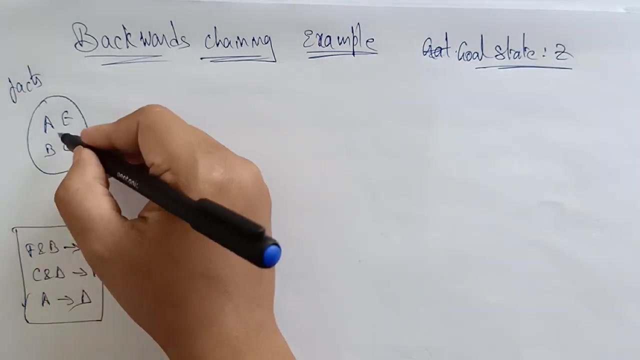 So here, this is a backward process. The backward process here I am taking: I want Z. Okay, because the goal is Z. The goal state is. goal state is Z, I want Z. Where is the Z? So from the facts there is. in the facts there is no Z, but in the rules the Z is there. I am processing in the 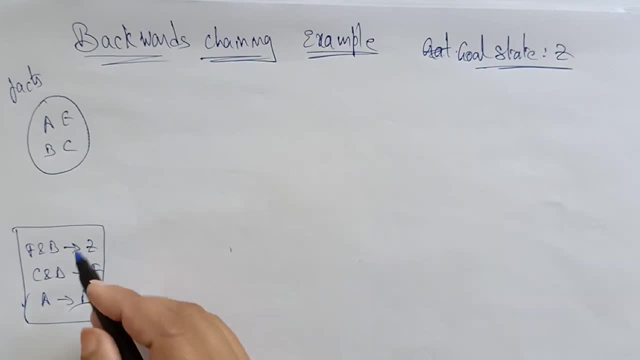 backward direction. So see the difference how in the forward I take in whatever they are matching: that element and that that elements matching, which implies the element, the remaining element, I am placing in the facts, that is, in the forward chaining, But in the backward chaining what I am 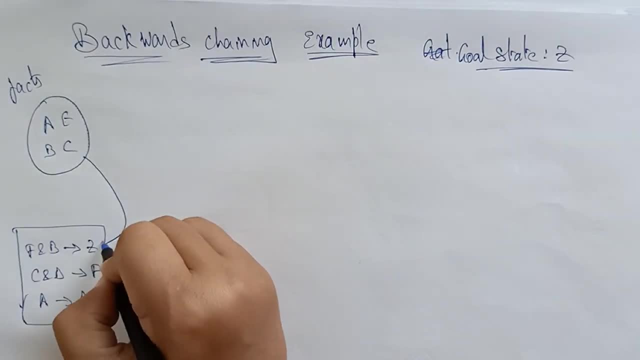 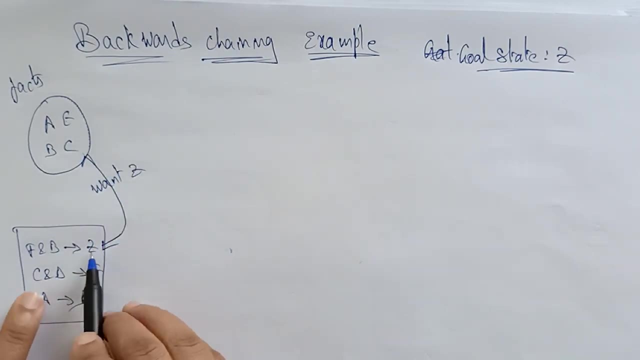 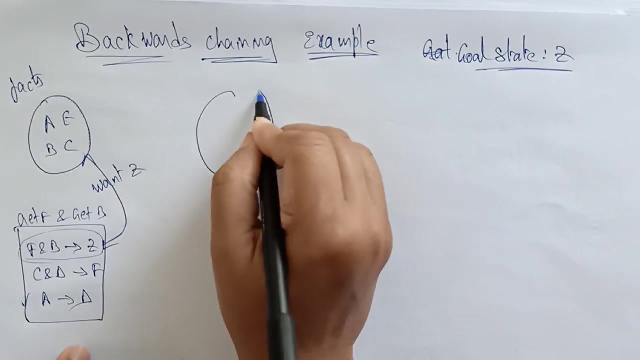 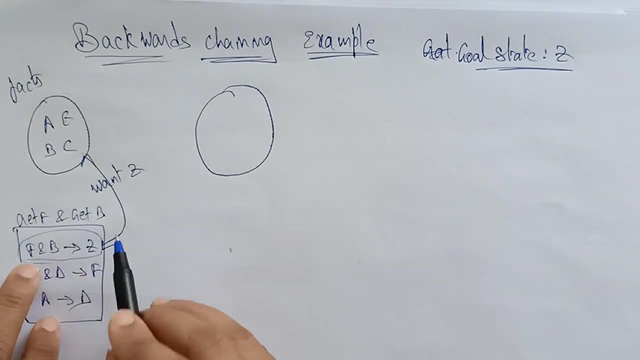 doing here is: I want Z. Where is Z? I am checking. Okay, I want Z, because that is my goal state. I want Z, So Z is present in this rule. So now I have to get F and get B, So next, get F and B, So next. whenever I say get F and B first, I am getting the. I want F. 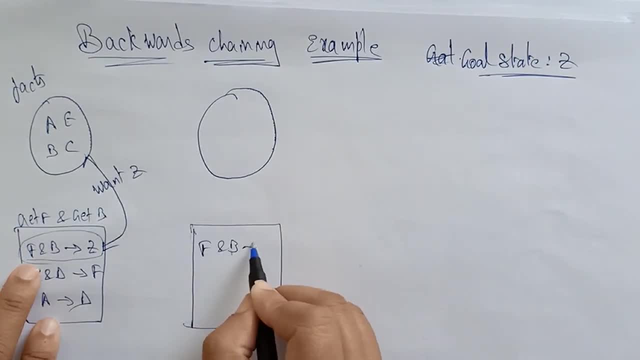 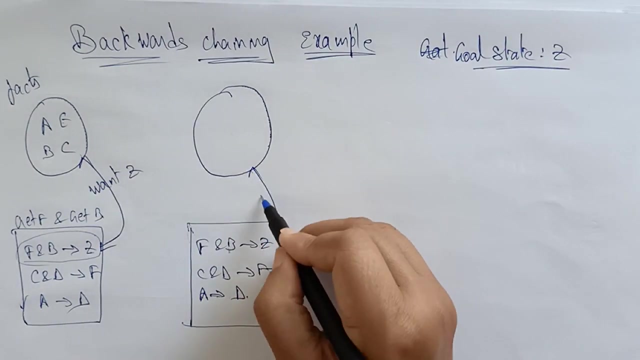 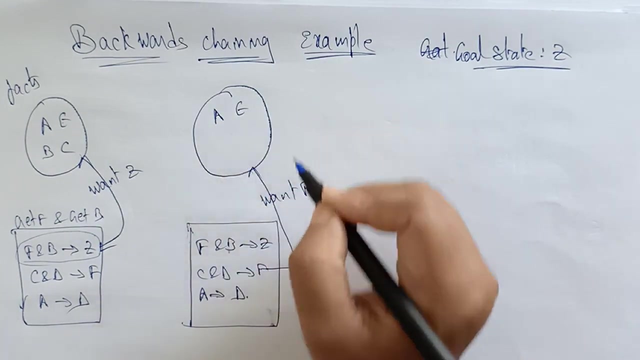 F and B implies Z, C and D implies F, A and D. A implies D. So now, this time I want F, I want F, Okay, So A, E. So whenever I want, F means what are the elements that are placed here? 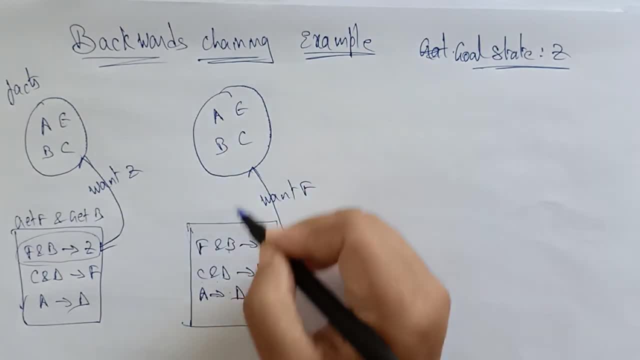 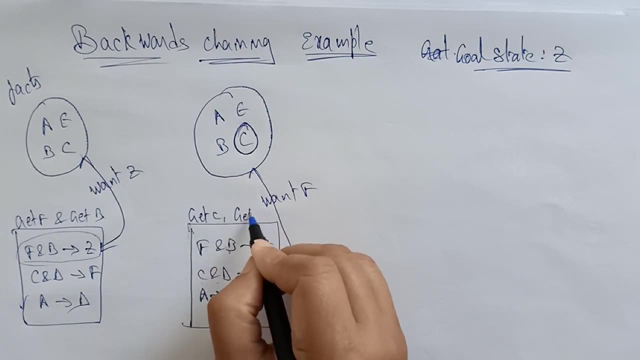 C and D is there. Okay, But C and D is not present. Only C is present. in the fact, The C is matching here. Okay, So get C, get D. So C is already matching here. Okay, C is here. previously, B is. 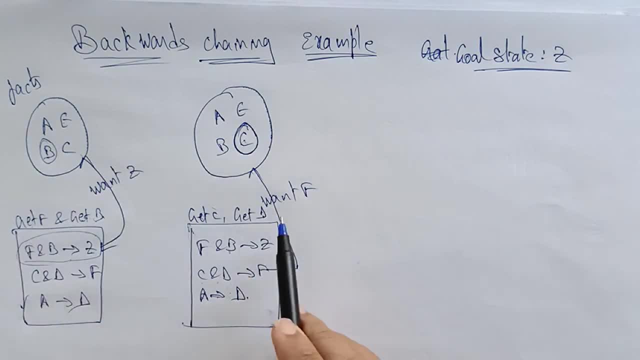 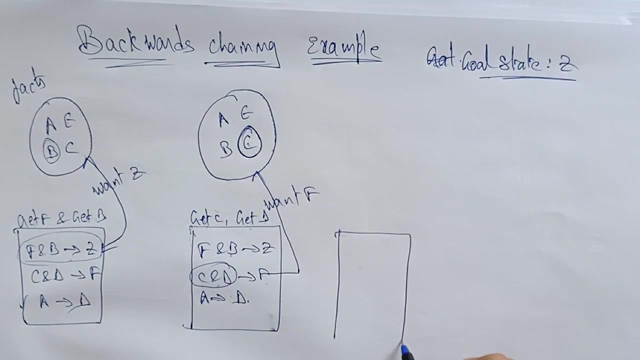 matching. So whenever the B is matching, I am just next time I am just taking. I want F, Okay. So, whatever the elements that are present, F is get C and get D. So C is already present here. So next I want which element I need to get. I want D This time. I want D, F and B because C 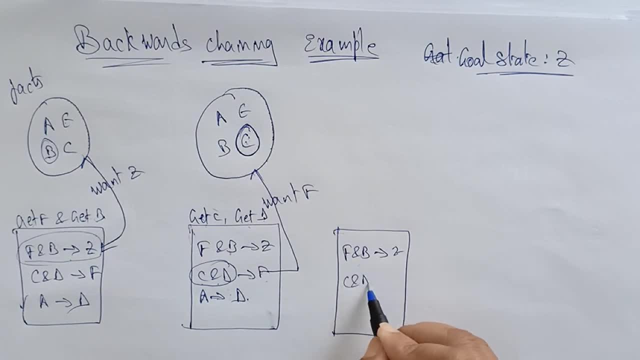 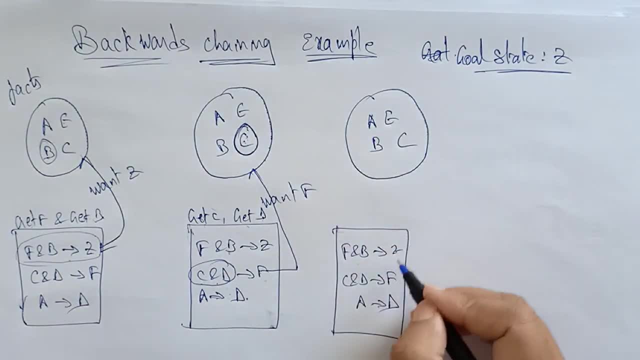 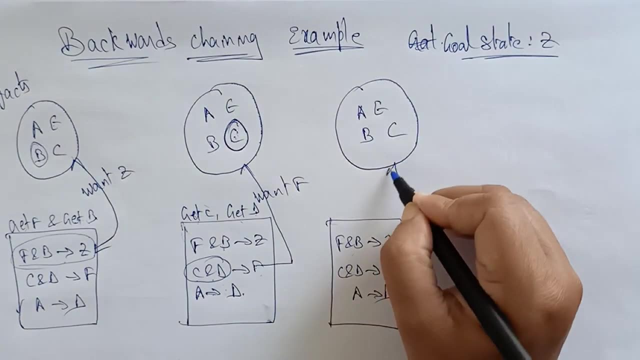 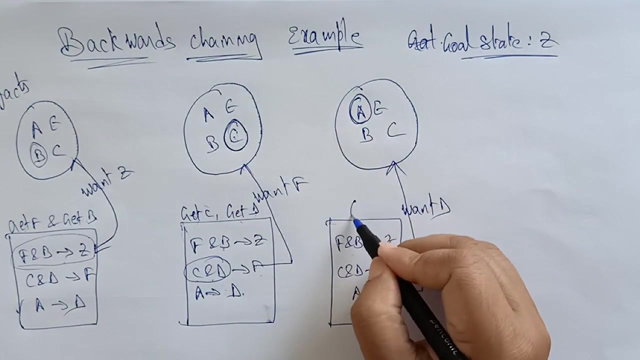 A, E, B, C. Okay. So I am asking: I want D. So where is D here? D is present here. I want D, So A. So A is already in facts. That is, get. A is already in the facts. So this is one condition. it is over. 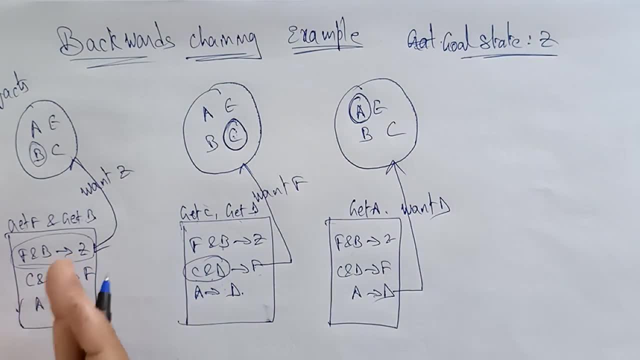 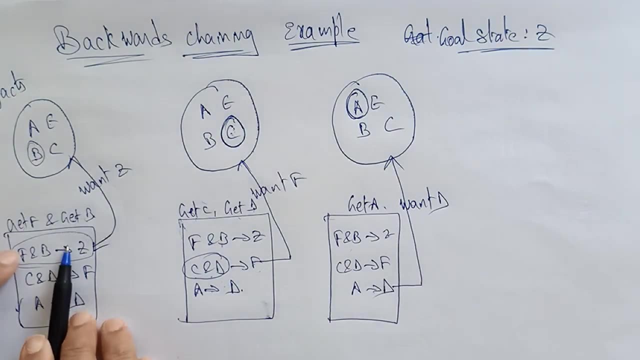 Now I started the execution because I get the elements of F, B, E. I get all the means from top to bottom. I reach every element, First the top. It is a top down approach. Okay, F and B: I executed. Next, C and D: I checked. Next, A and D: I checked. Now I want to execute. So take this element. 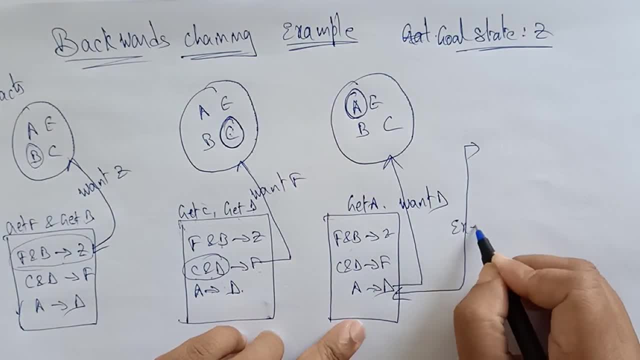 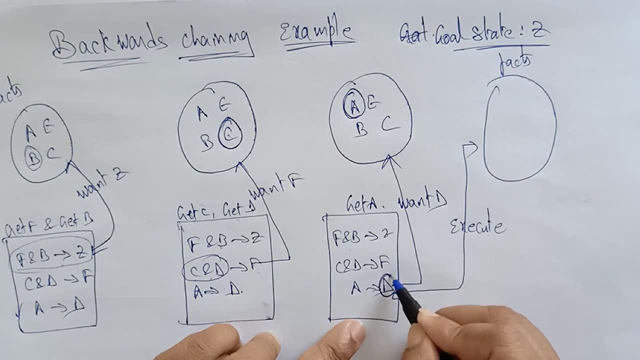 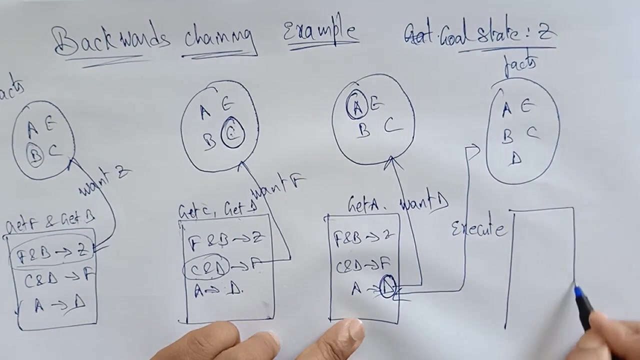 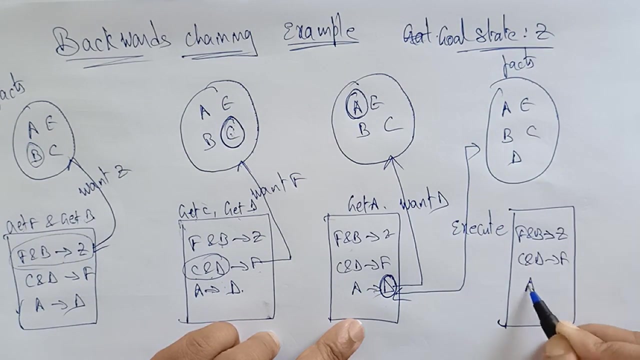 and start execute Means. you have to place that in facts, In the facts you needs to be placed. So what element you have to place? The D has to be placed A, E, B, C, D, Okay. So now follow the same process. whatever you have done in this forward. F. A implies D, Okay. So D and C. 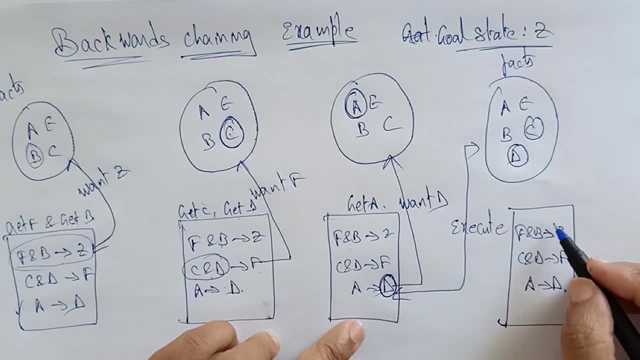 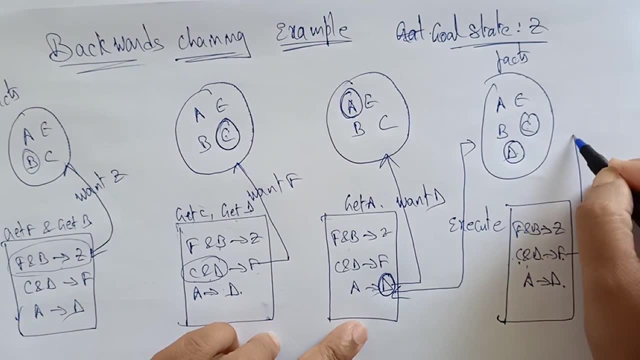 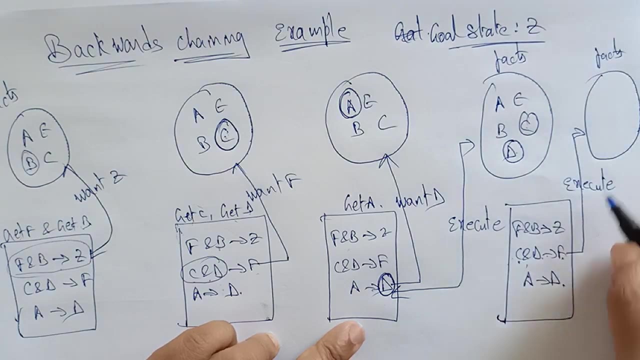 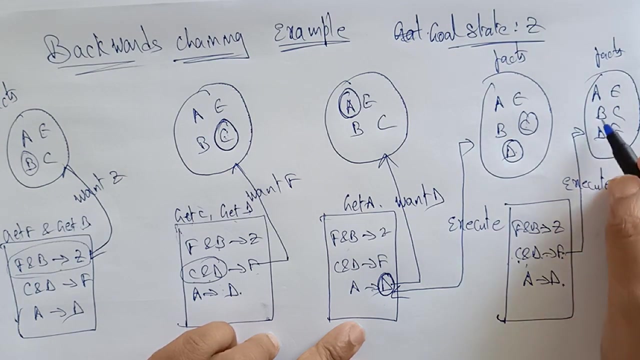 So already C and D is here. is there Means I want to execute now F. What is the C and D combination? So these are matching. The C, D is matching to this rule. So I need to execute F. Execute FATs, So F I need to be execute here. A, E, B, C, D, F. Okay, So F contains F. I executed. 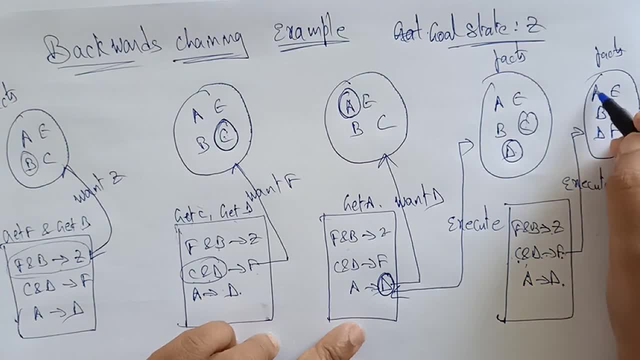 Now check which rule is matching. F and B is matching. Okay, Because F and B is matching with the rule. So this time F and B implies Z, A implies D or C and D implies F. So F and D is matching. A implies B or C and D implies F, So F and B implies C and D, So F and D implies C and D, So F and D implies 9.. So F and B implies O or C and D implies F, So H. Okay, And now I repeat this one おこりne primary action there.